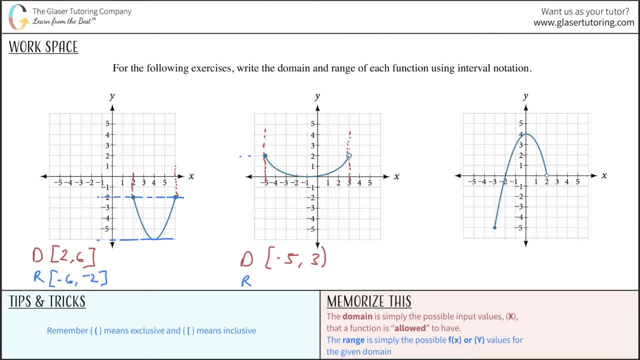 just as easy. right, It goes all the way the function. the highest point is going to be two and the lowest point that the graph obtains is going to be zero for y. that is so, and they're both inclusive of those points, and therefore we could say: now the 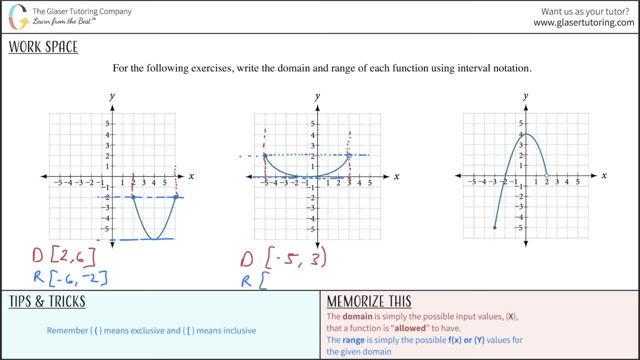 range is going to be inclusive of two. well, actually, i'm going to start least right, inclusive of zero, all the way to two inclusive, all right. um, then, taking a look at the next one, okay, we now have, uh, the leftmost point is going to be x being negative three. okay, and then it goes all the 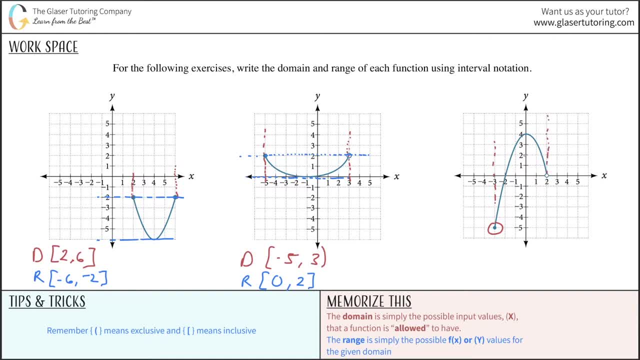 way on out. the rightmost point is going to be two, but not inclusive. so how do we write so simply? how do we uh mark that down? so the domain here is going to be all the way from negative three, inclusive of it. that's why i have the bracket all the way to two exclusive. so that's why the 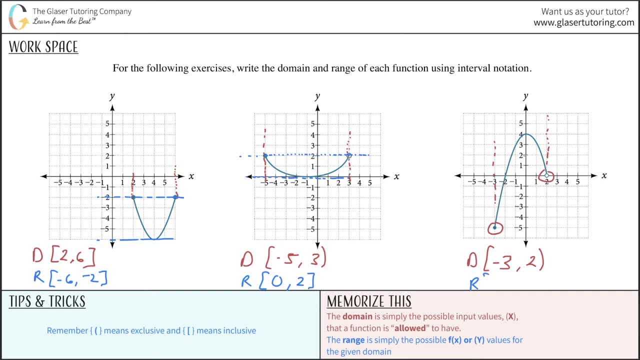 parentheses and then the range. now we're thinking about the lowest to highest values. actually, let me leave out the bracket for now. the lowest value that this function obtains is going to be five and the highest value that this function obtains is going to be four right, negative five, i hope i said if i said five i meant negative five. all right, so from negative. 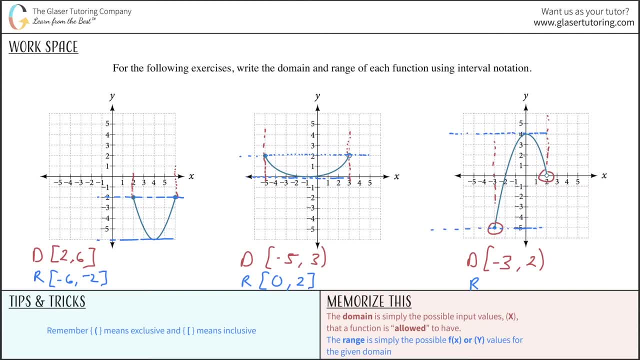 five all the way up to positive four and inclusive of those points. so, uh, we have a bracket here. it's going to be negative five, uh comma, then uh, four inclusive. okay, just also a note on this one. i'm thinking about it. um, you know, when i drew my horizontal line here, you might say, well, it. 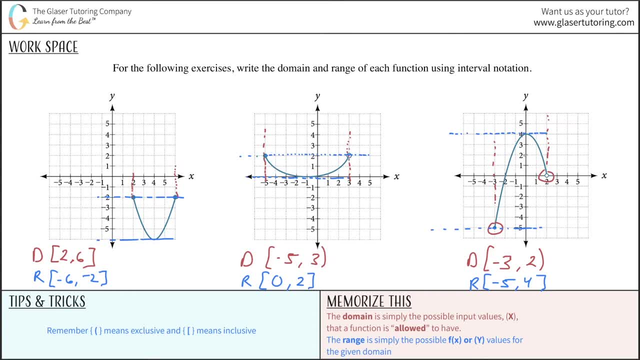 includes this point, but it doesn't include that. so can i say that the the range goes all the way up to two and yes, we can. since it includes one of them, right, doesn't have to include both. as long as this function here, this graph, reaches two at some point, it reaches two over here, then we that. 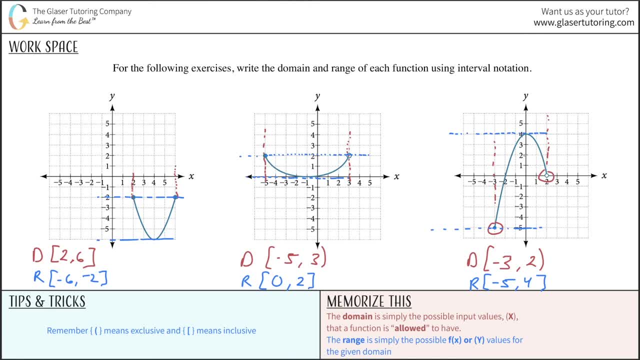 is part of the range. that's the highest point that the graph reaches. all right, just to clarify that. guys. thanks for tuning in. please remember to subscribe. see you next time, take care you.